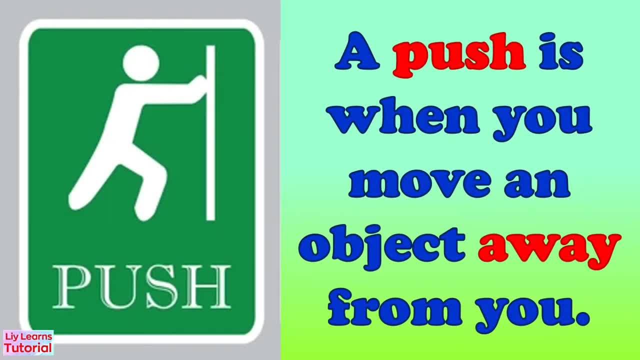 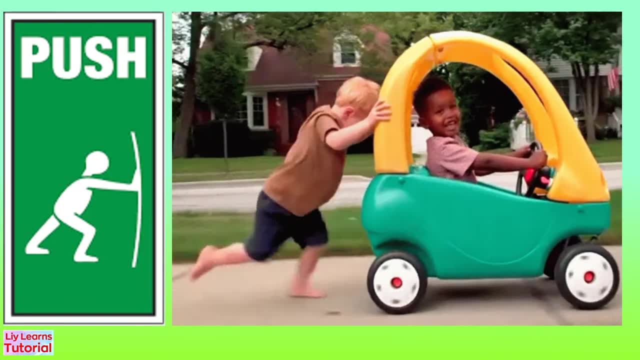 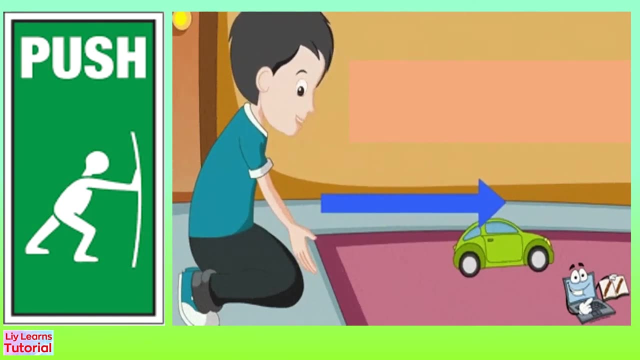 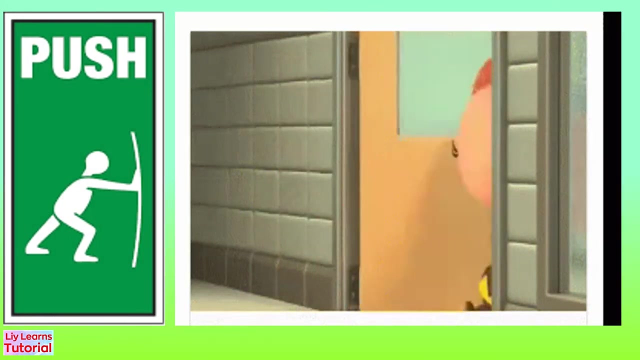 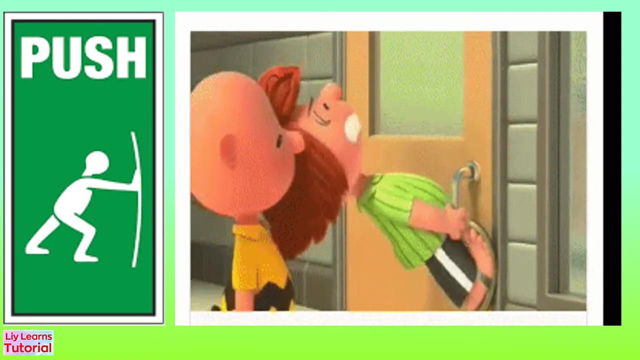 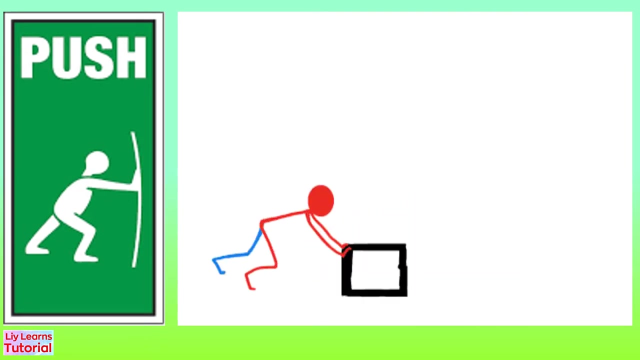 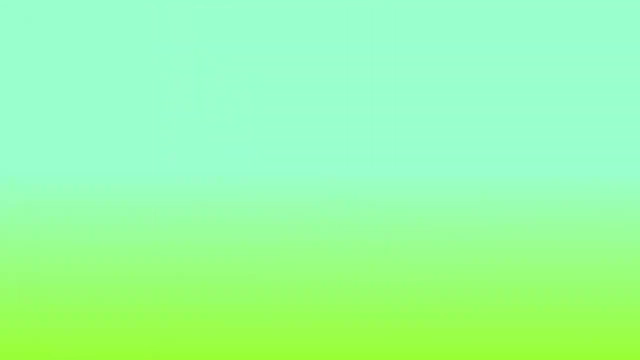 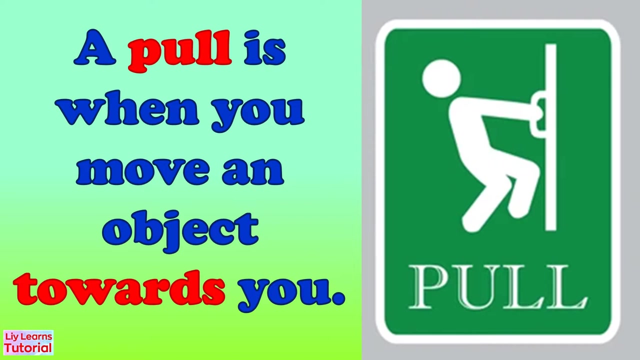 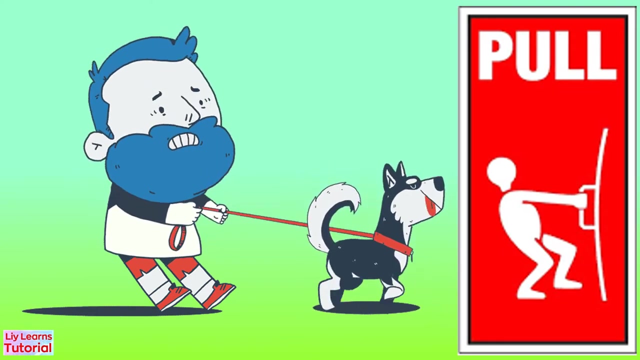 A push is when you move an object away from you, Like this one, Pushing a toy car away from him, Pushing the door, Pushing a box. A pull is when you move an object towards you. This is an example of a pull. 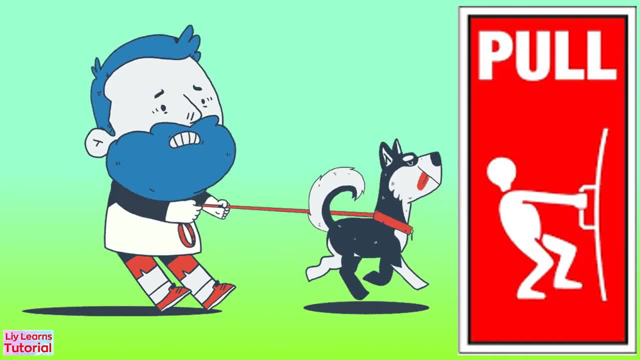 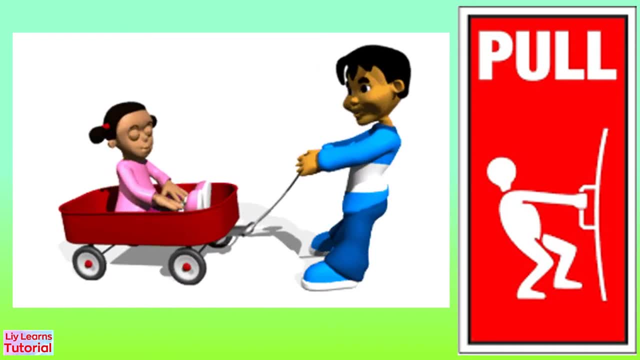 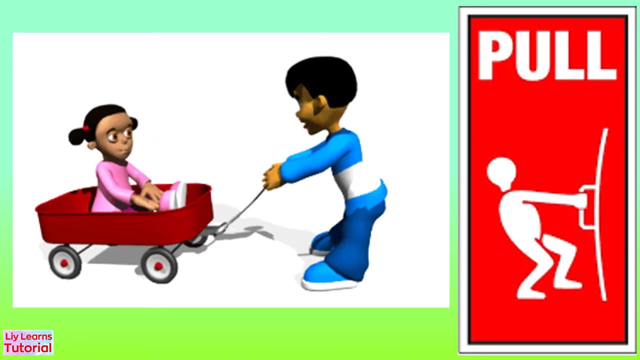 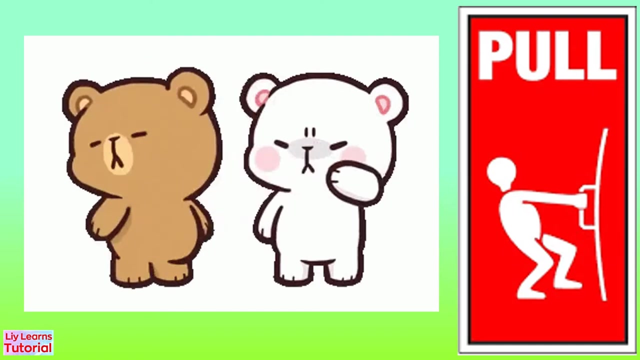 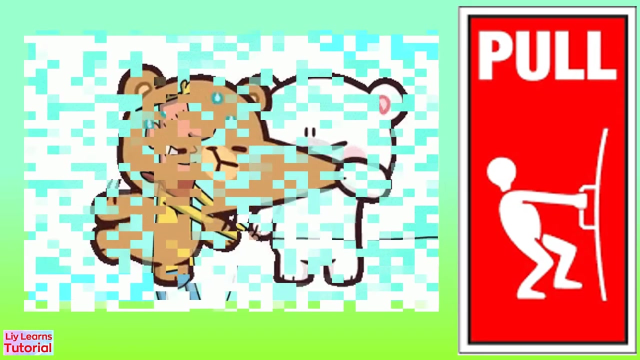 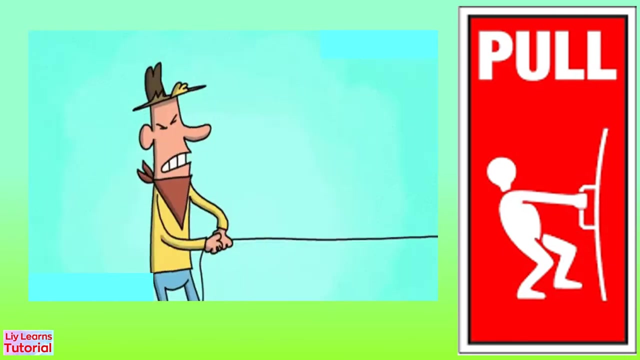 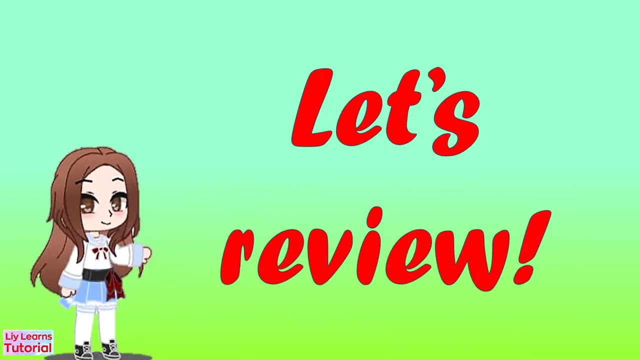 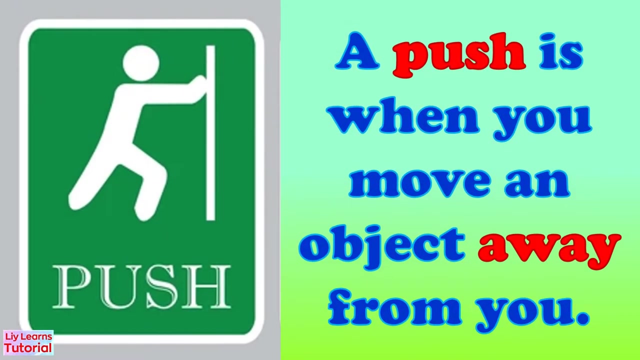 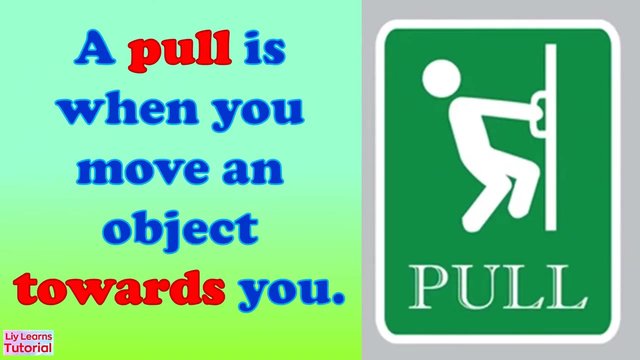 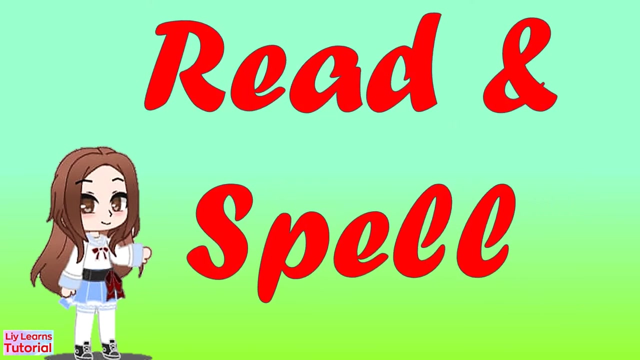 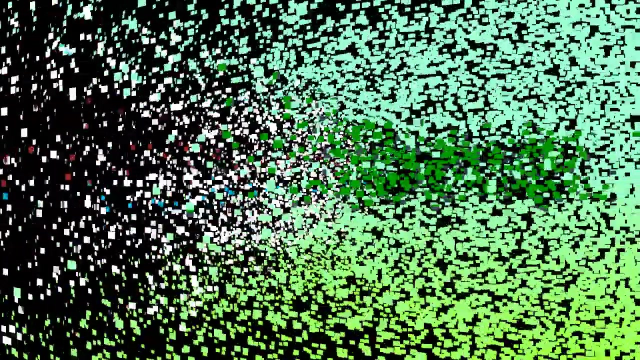 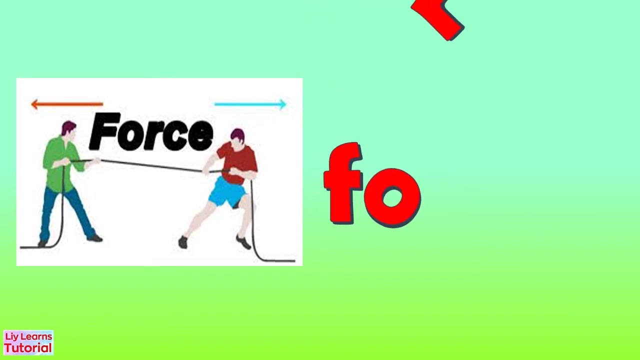 A lift, Pulling the cart towards the boy, Pulling the cheek, Pulling a rope towards him. Let's review: A push is when you move an object away from you. A pull is when you move an object towards you. Let's read and spell: Force, Force. 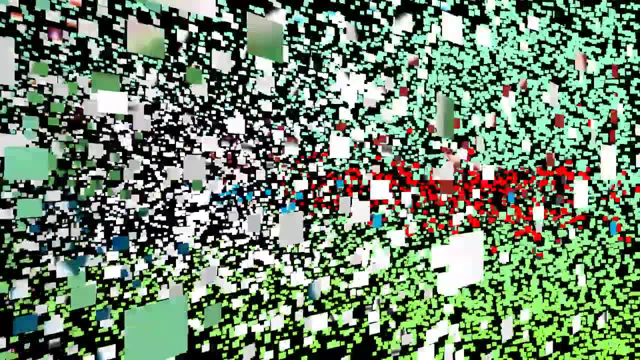 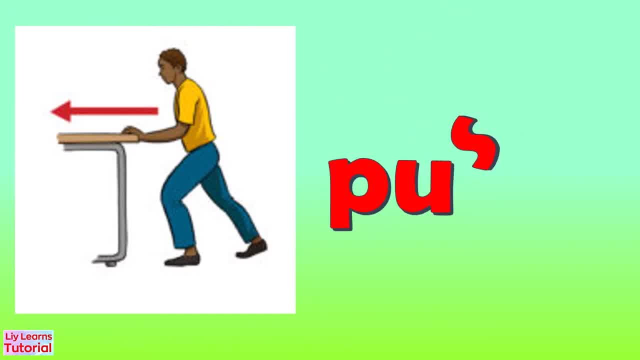 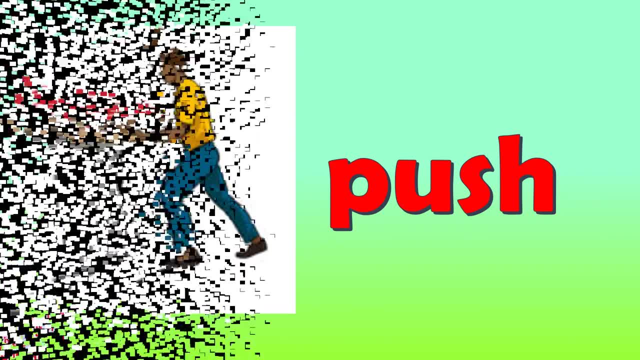 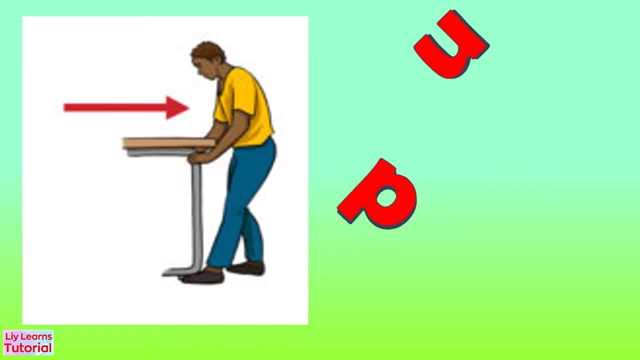 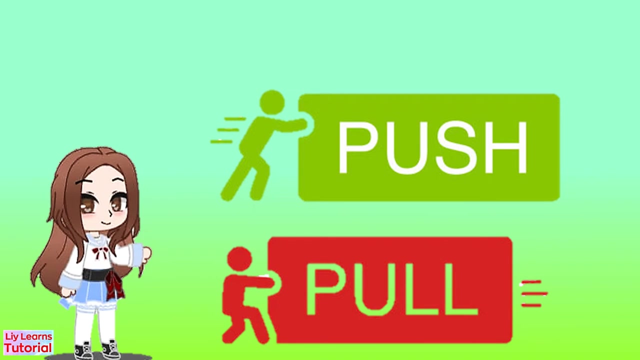 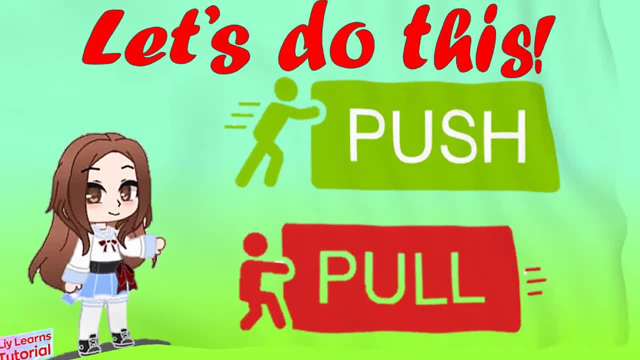 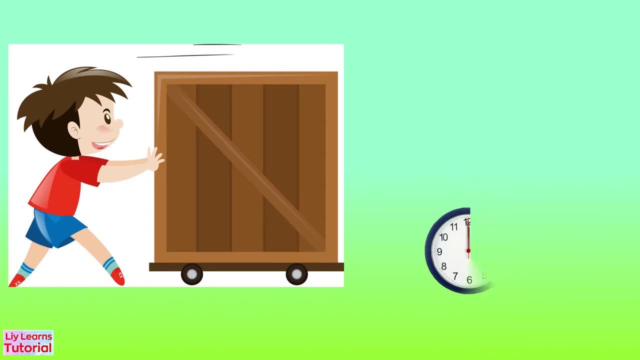 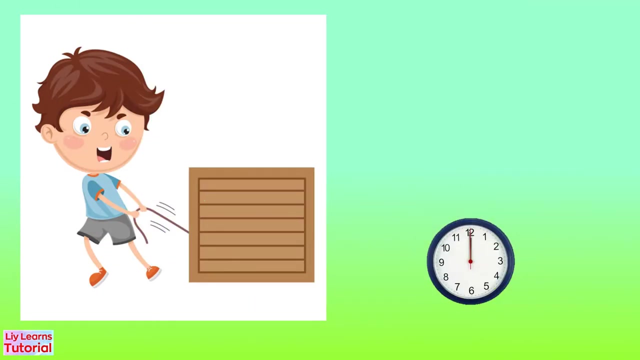 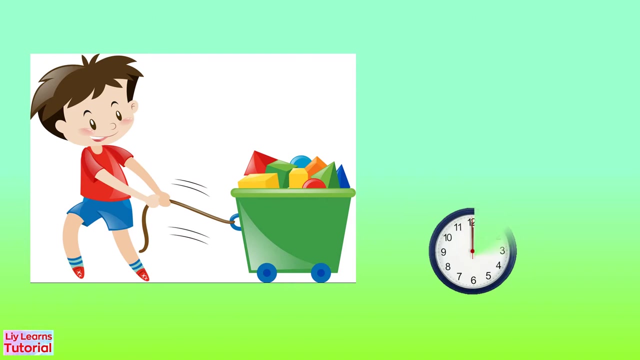